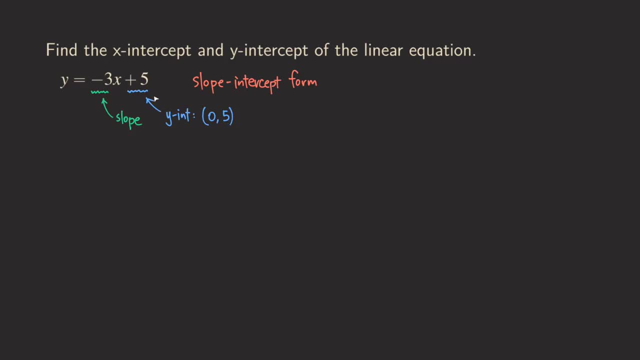 have the y-intercept without any calculation. So that's the benefit of writing the equation in the slope-intercept form. Okay, so we already got one answer. Now you may say: what about the x-intercept? Now, the x-intercept is something that we need to do: a little bit of calculation, Okay, and to find 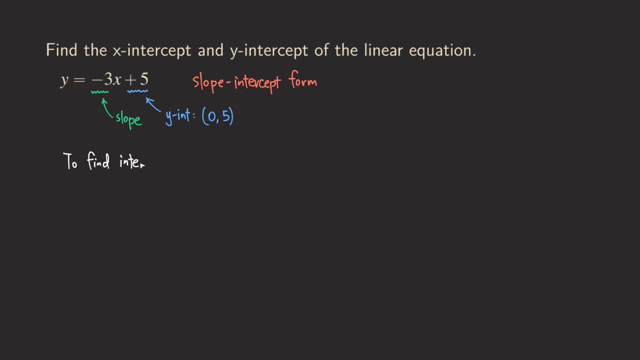 the x-intercept. what happens? Okay, so we need to find the x-intercept. What happens is that we are going to do what. Here's the idea: We are going to set y equal to zero, and then you may say why do. 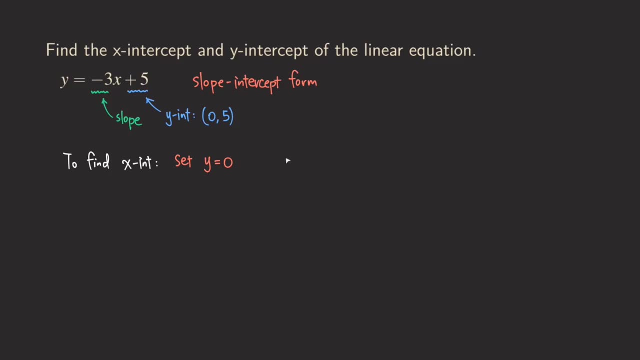 we do that. It's really because when we set y equal to zero, okay, then that is where you just look at the xy-plane and you try to grab this line right here. okay, When y is equal to zero, we are actually. 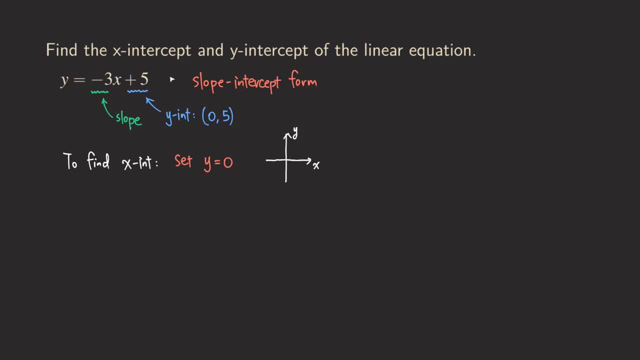 looking at a point on the x-axis. That's where the graph of the line is actually intersecting They x-axis, So that's how we find the x-intercept okay, And so, of course, for this line, for this. 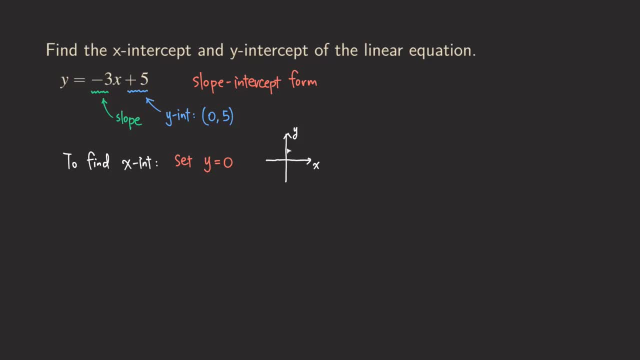 line. we have the y-intercept, which is 0,, 5,, right So, and then it has this little bit negative 3, so the line is actually looking like this. This is really just a sketch for this line, It's not. 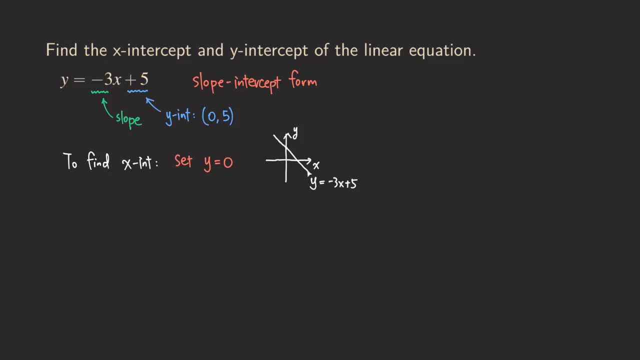 too accurate, but then I'm just going to show you what it looks like. And now we already figured out this y-intercept right here. which is what? Which is 0, 5.. That's the y-intercept, The x-intercept. 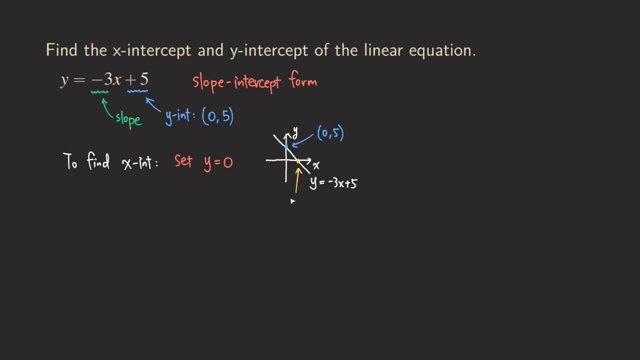 okay, The x-intercept is this one, And, as you can see that the y must be 0 in this case, okay, And now the question is: how do you find the x? And so we've got to do the calculation, okay, So. 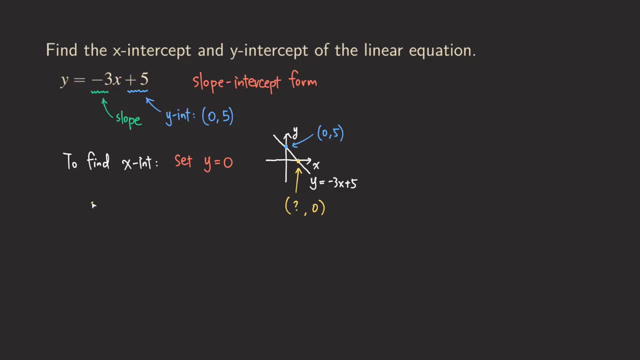 once we set y equal to 0, then we are going to get what We're going to get: 0, okay, Because the y becomes 0. And then now we still have negative 3x plus 5.. And so this is the equation. 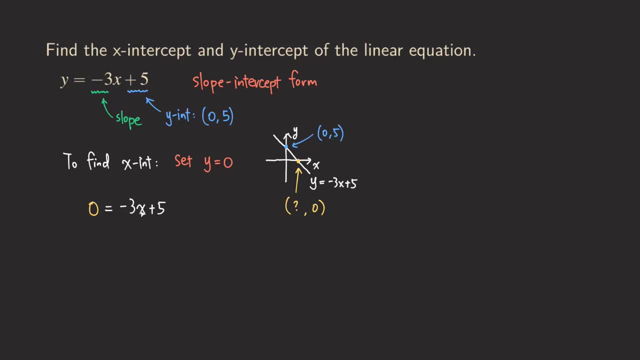 that we're going to solve, And it's actually easy to solve because there is- it's the same- the equation with x being the unknown. So we just need to isolate the x here, So moving the 5 over. so we're going to subtract 5 from both sides. So we are going to subtract 5 from both. 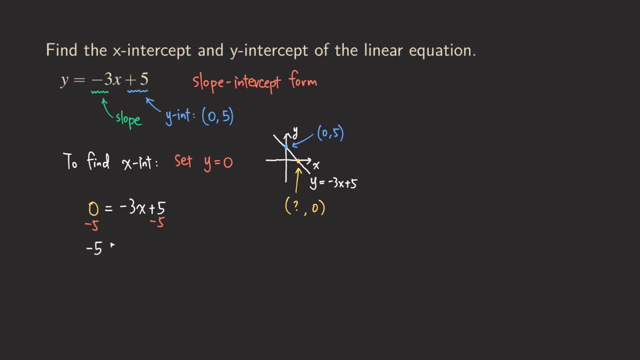 sides, okay, And then what happens Then? we are going to get negative 5 equals negative 3x, okay, And then isolating the x means that we get a. what We get to divide both sides by negative 3, because it's multiplication, right? So divide both sides by negative 3 here, And then we are. 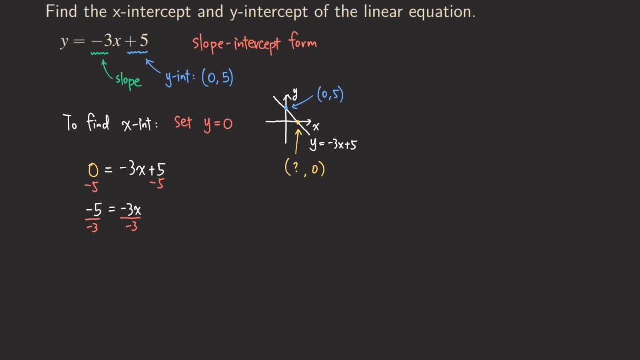 going to get what? We are going to get negative 3 plus 5.. And then we are going to get negative 3 over negative 3.. The negative signs will get canceled, So we get 5 over 3.. And then what do? 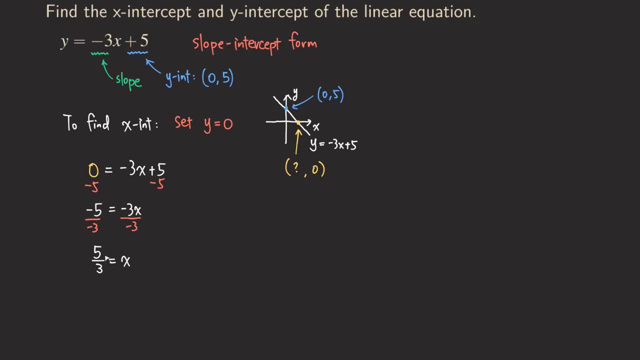 we get here, The negative 3s will get canceled. So we just get x, And so we already figured out the answer. So what can we say about the x-intercept? Now we go back here and then we 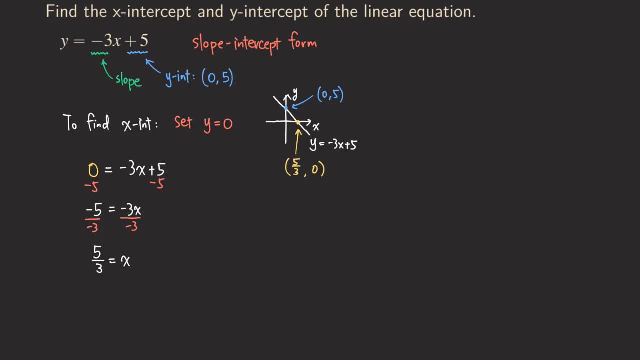 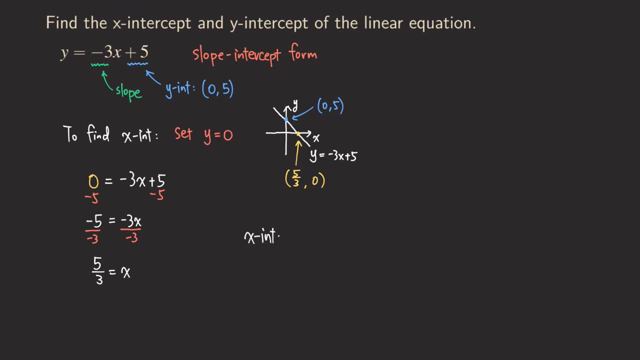 write down the answer. So we get 5 over 3x as the x-intercept. So right now it's actually good to start writing down the answer. So the x-intercept, okay, is going to be what? 5 over 3 and then 0.. And then what about the y-intercept? The y-intercept. 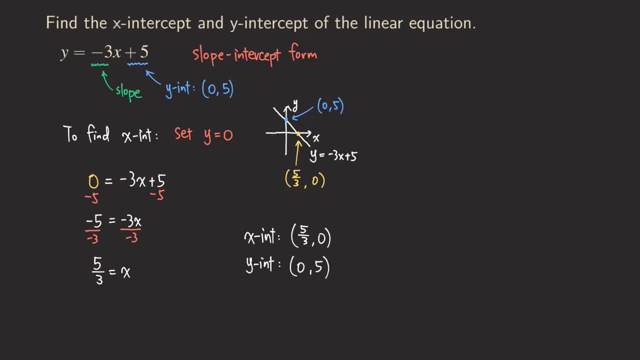 is going to be what? 0, 5.. So we have the final answer. Okay, So that's it for this problem. We are going to see another example next time. Thank you for watching. I will see you. 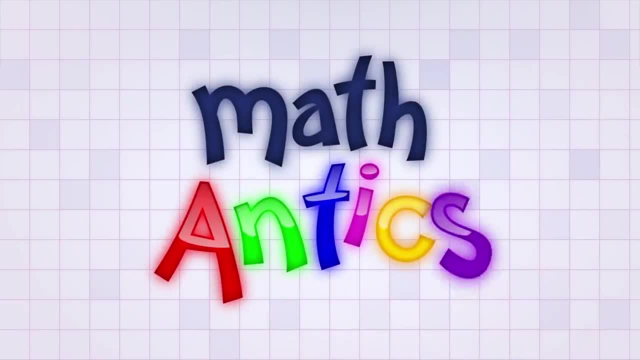 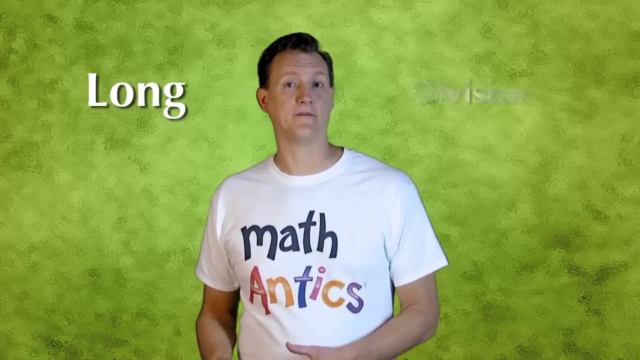 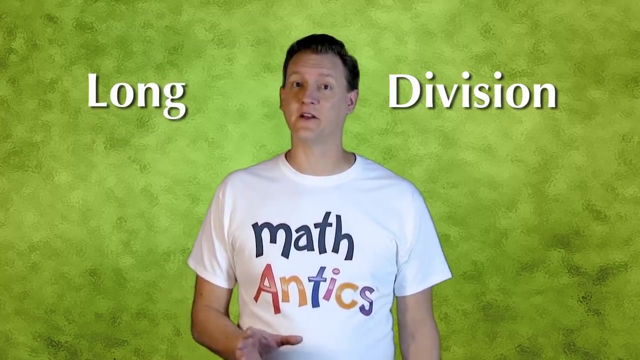 Hi, welcome to Math Antics. In this lesson we're going to learn about Long Division. If you haven't already watched our video about Basic Division, then be sure to go back and watch that first. It'll make learning Long Division a lot easier. 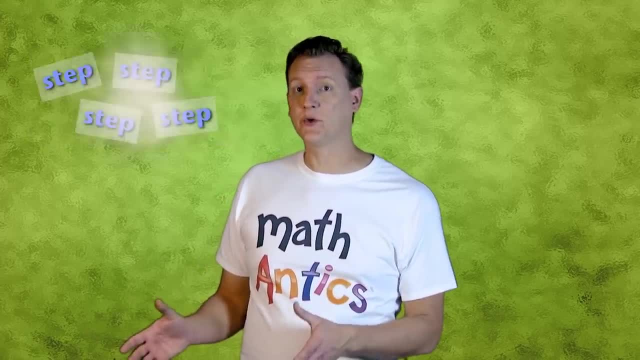 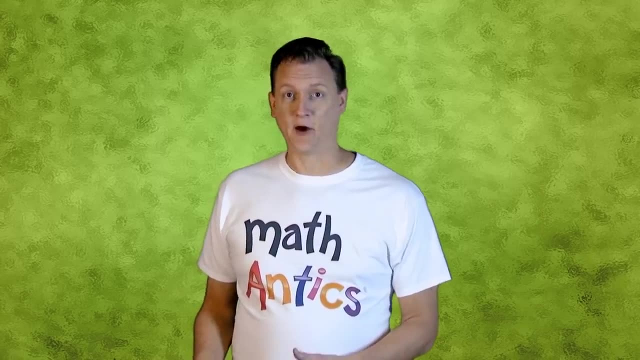 Long Division is just a way of breaking up a bigger division problem into a series of short division steps, like the ones that we did in the Basic Division video. The nice thing about Long Division is that once you know the procedure, you can divide up all kinds of numbers, even if they're REALLY big.